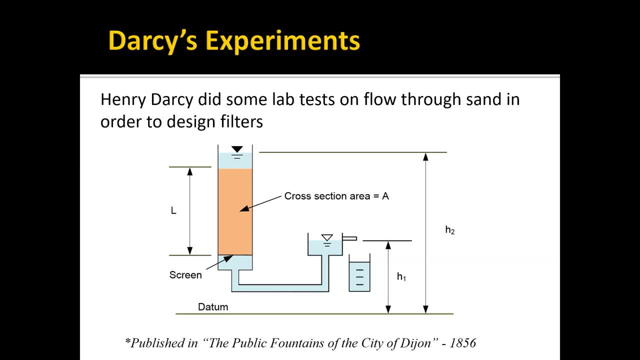 Now imagine if you're trying to design a filter as an engineer and you need to determine how much water- excuse me, you probably start out with knowing how much water you can pull from your reservoir in terms of a flow rate, cubic meters per day, something like that. 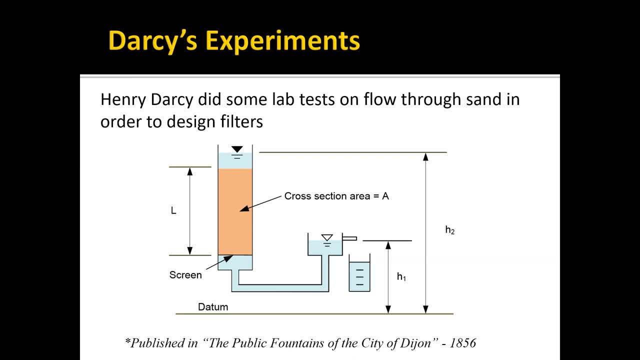 And then you have to design a filter. They understood the concept of hydraulic head and how you get head loss as you move something through a filter, And the finer the material, the more the head loss you get. But they knew they had to make the filters a certain size. 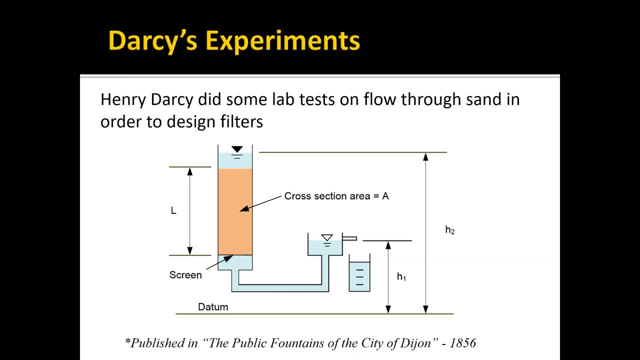 They knew they had to make the filters a certain size and length. But how do you go about doing that? And so Henry Darcy did a series of tests in a laboratory, where he took columns of soil, as shown here, and had water fed into one side, and the water coming in was maintained at a certain 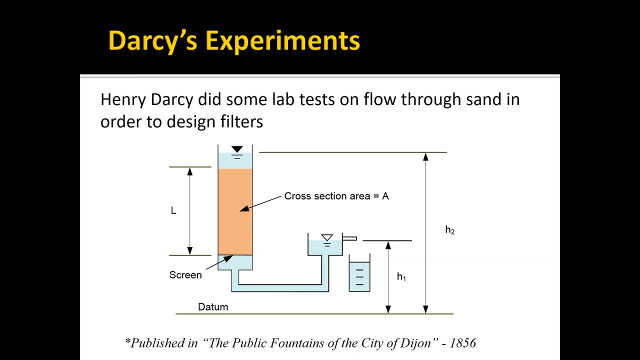 head, which we'll call head two here, And then the water would go through the soil, which would act kind of like a filter. And then the water would go through the soil, which would act kind of like a filter. there would be head loss as that happens, and then it would be drained off into a 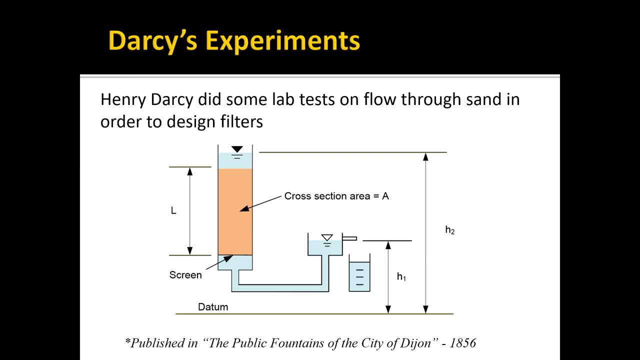 into some sort of container. There was a little spout that would maintain a consistent head or water level on the downstream side And he would also vary the length of the column of soil in the cross-sectional area and vary the the head difference as well. 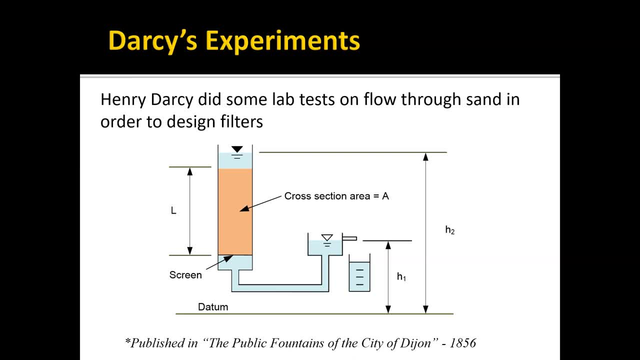 And record how much water would come into the cup. So what, what kind of volumetric flow rate would you get through this system over a certain period of time? These experiments were published in a book called the Public Fountains of the City of Dijon in 1856.. Some of these experiences were: 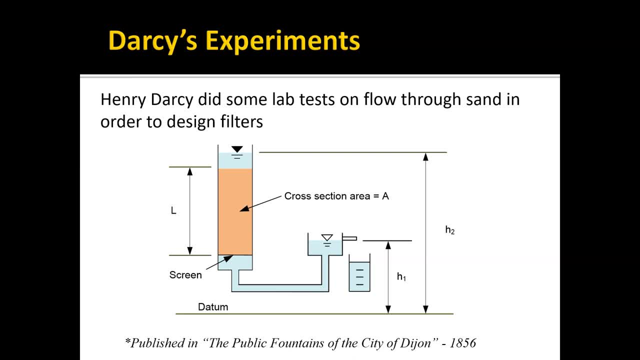 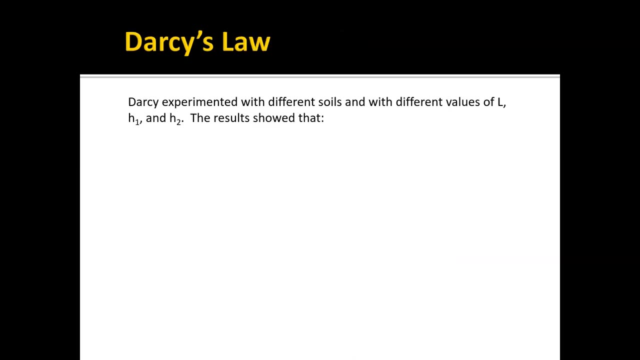 done in the 1830s, all the way up through 1856. And he based all of his findings on programs, things wereätz. Based on these observations and these tests, he came up with a simple equation which we now call Darcy's Law. 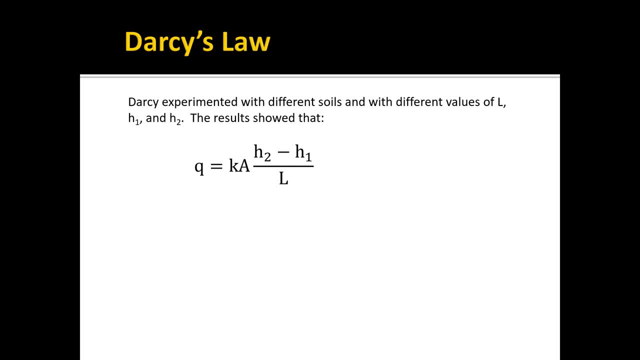 So Darcy's Law is: Q is equal to Ka times H2 minus H1 over L, where Q is equal to the volumetric flow rate, the volume of flow that goes through the soil in a certain period of time. So this would be like cubic feet per second, cubic feet per day or cubic in this case. 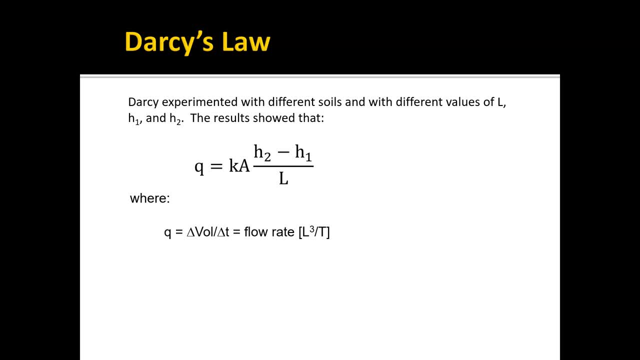 I'm sure it was cubic meters or cubic centimeters over a certain length of time, and that's how much water is going through the system. The term K is a constant that is a function of how permeable the soil is, so it's called 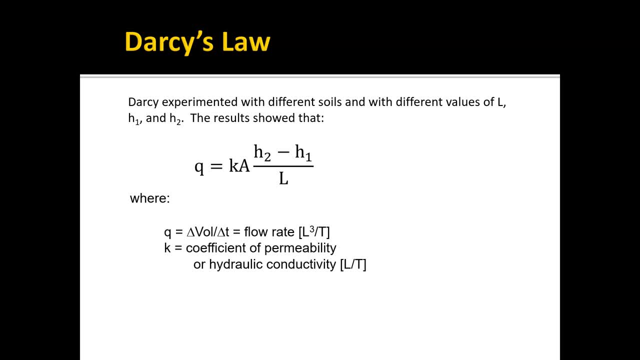 the coefficient of permeability. A is the gross cross-sectional area of flow of the cylinder, and when we say gross we mean not just the soil area but the water area, just the entire area cross-sectional area that's flowing through. We'll come back to that. 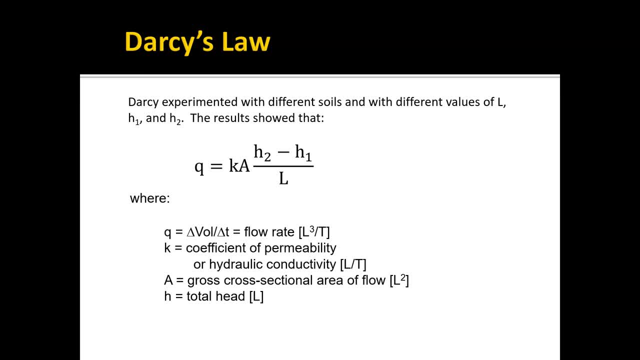 H is equal to total head and H2 minus H1 is the head difference. The flow rate is the length of the flow path that it goes through. So let's think about this for a second. So what this says? if you look at it, it's just a simple algebraic equation. 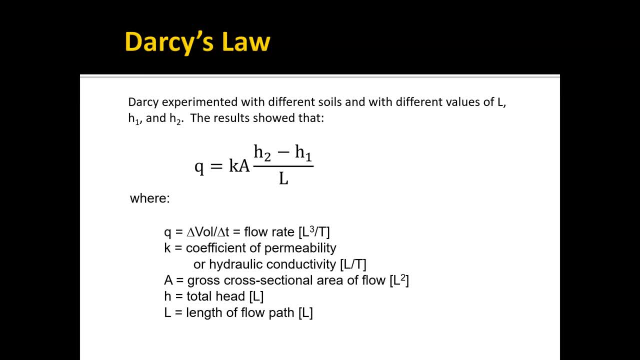 The greater the cross-sectional area, the more flow you have. So the flow is linearly proportional to the area. That should be intuitive. The bigger pipe, bigger flow. So you can see that, You can see that. And then, since the H2 minus H1 term is on the numerator, that means the larger the head. 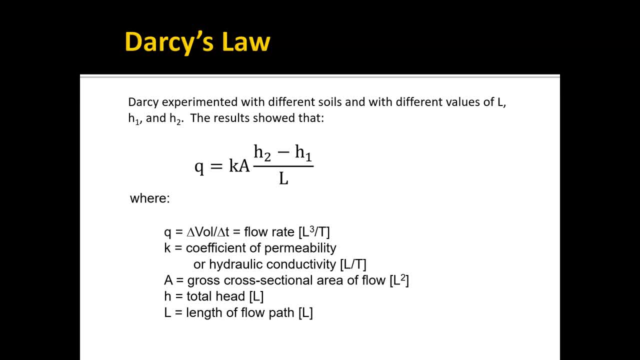 difference, the larger the flow. Those are linearly related. and then the length of the column is in the denominator, So the flow is inversely proportional to the length of soil that it has to go through. Since it has to travel, the more energy it takes, and so for a given head difference. 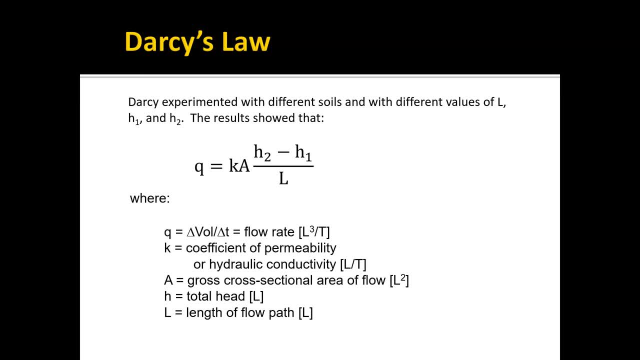 if you double the length, you're going to reduce your flow rate by half. And then finally, this coefficient K. we determine that experimentally using a test much like the one shown on the first slide And that has units of length per time. 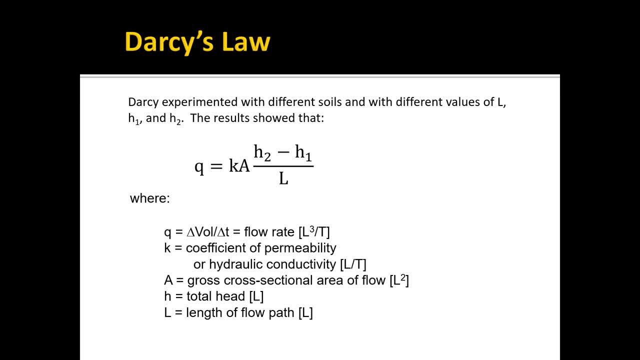 So centimeters per second, meters per day, feet per day, And that is a function of how permeable the soil is. Gravel, for example, would have a very large value, and sand or clay would have a smaller value. So that is Darcy's Law. 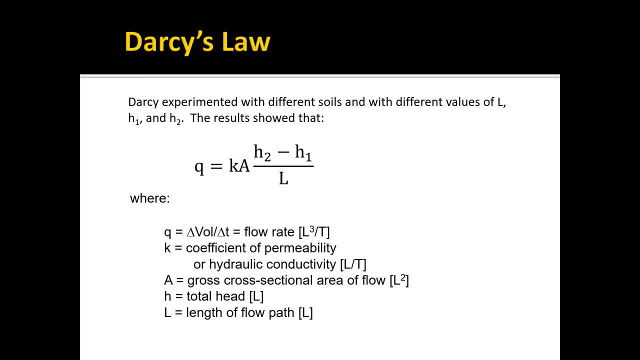 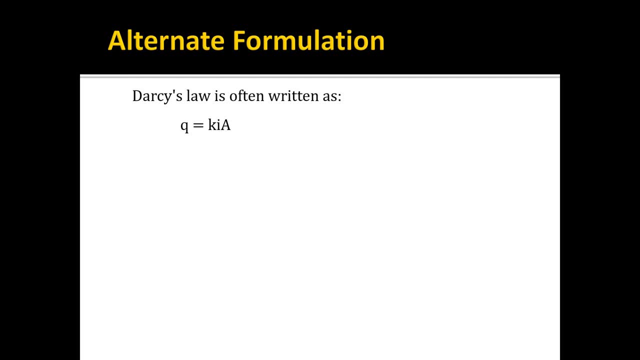 Should be kind of intuitive. It makes sense. The beauty of it is it's very simple, And sometimes you will see Darcy's Law written in this form. It's called the I-A And what's been done here is the I term is called the hydraulic. 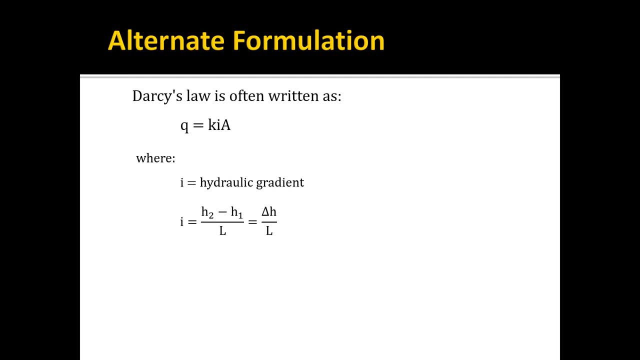 gradient And we've just lumped the head change divided by L into a single term, So it's the change in head divided by the length. It's called a gradient because it represents how rapidly the head is changing Versus distance. And the greater the hydraulic gradient, the greater the flow rate. 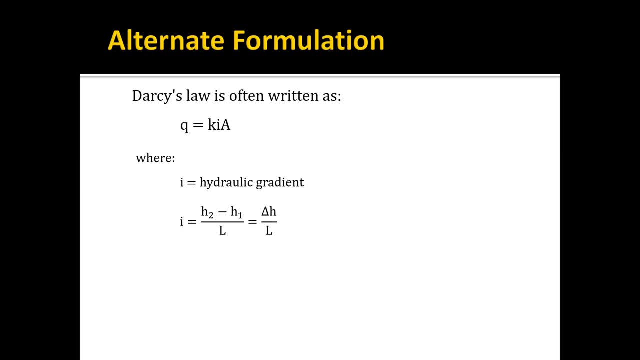 It's linearly proportional to the hydraulic gradient. This can also be written in derivative form as minus dh ds, And sometimes you will see Darcy's Law written in this form. In fact, when we go through our governing equation derivation in one of our upcoming 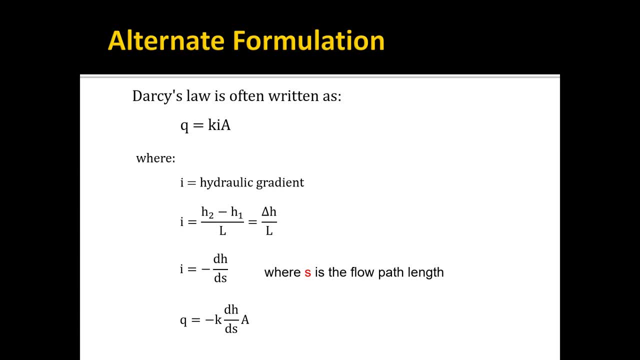 lectures. this is actually the form we will use. So dh ds means it's the hydraulic gradient. It's the hydraulic gradient. It's the hydraulic gradient represented as a derivative. Now, the minus sign is important here, because if you look up above this, h2 minus h1, it's 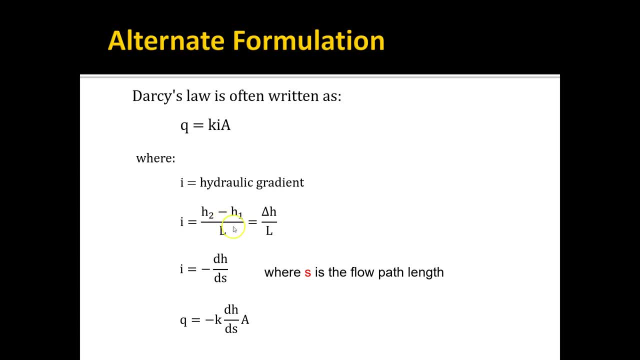 basically the high head where it starts minus the low head where it finishes is the change in head. But when you do a derivative it's typically The head you end up with minus the head where you start. So if you go from a high head to a low head, this derivative dh ds would be negative. 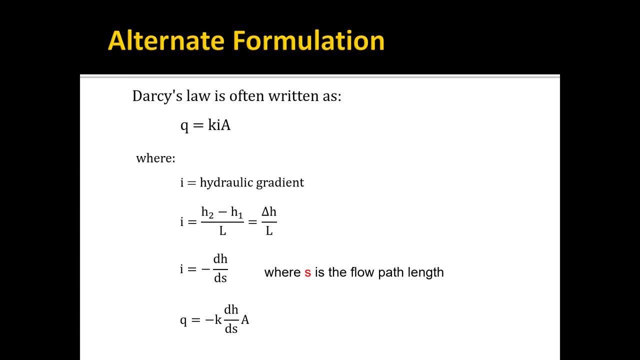 And we put the minus sign on there, because water flows from high head to low head, So it flows in the direction of maximum negative gradient And so, in order to You know, a positive flow rate would mean you know water flowing in a certain direction. 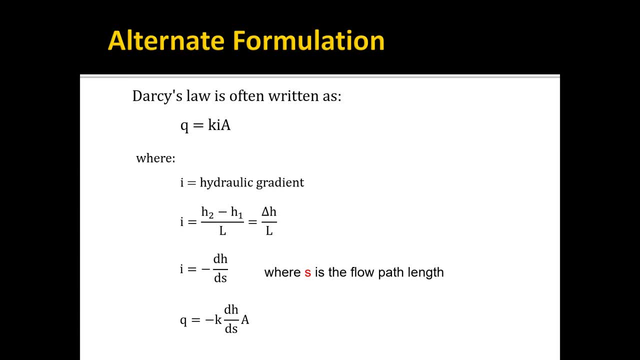 And so, in order to You know, a positive flow rate would mean you know water flowing in a certain direction. And so, in order to You know, a positive flow rate would mean you know water flowing in a certain direction. 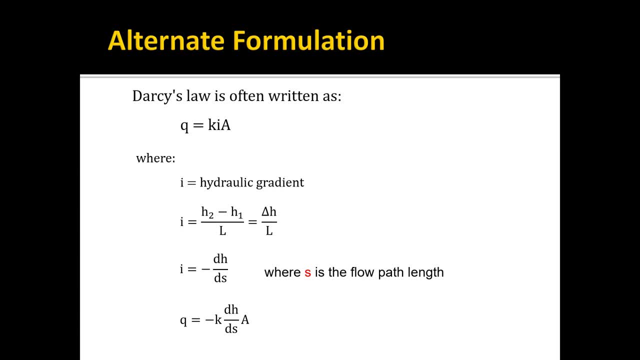 And so to get the sign to work out, we have to put a minus sign on. So if you see the derivative form, we use a minus sign. If you're just lumping delta h in there, we just make sure that we have the proper. 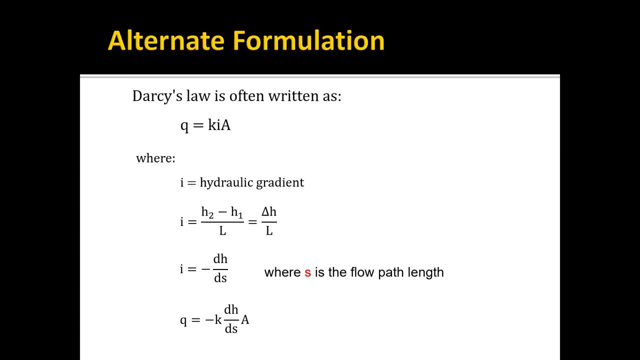 We've done it in the proper order to make it positive, But these are both very common representations of Darcy's Law. There's another way we can write Darcy's Law. There's another way we can write Darcy's Law. There's another way we can write Darcy's Law. 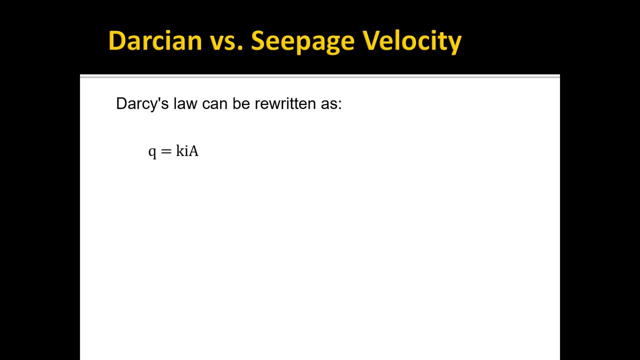 If you take q as equal to k, i, a and divide both sides by a volumetric flow rate, divided by area equals velocity, And on the right side the areas cancel And you end up with this term: vd equals ki. Sometimes they put the d subscript on there. 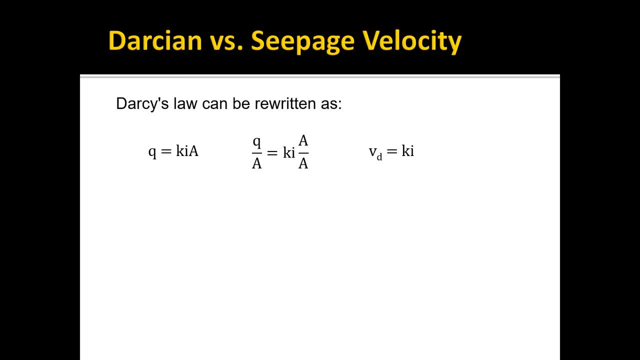 Sometimes they don't But the d. So basically vd equals ki. sometimes you see this: the flow velocity in porous media is equal to the hydraulic conductivity multiplied by the hydraulic gradient. So what does this mean? We've got to be careful. 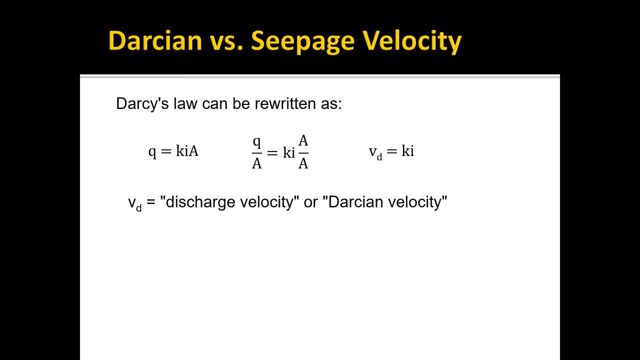 It's tempting to think of v as the speed at which water is flowing in the soil, but that's not quite right. Remember: what we've done is we've taken this column of soil, I'm laying it on its side And we're taking the total flow rate and dividing it by the full cross-sectional area. 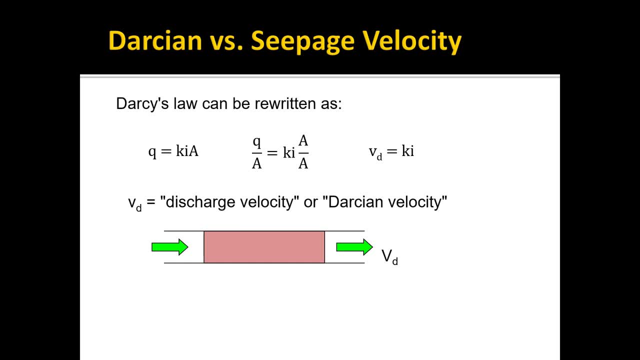 So basically, the Darcy velocity is how fast the water would be flowing in the empty pipe on either side of the soil. Again, if we take the total flow rate and divide by the total area, you're getting the flow in the pipe. That's really important. 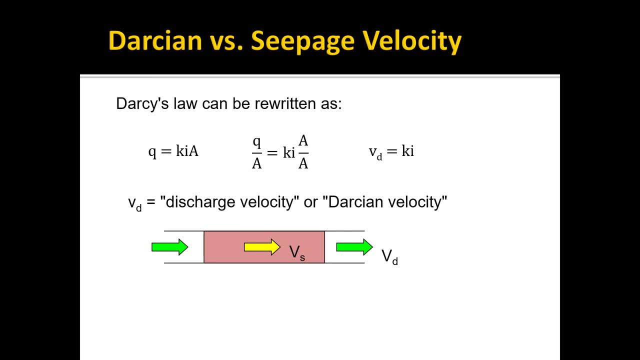 In contrast, the water that flows in the soil itself flows at what we call the seepage velocity. And why are they different? It's because the water that's flowing through the soil is going through just the pore space, the void space, in the soil. 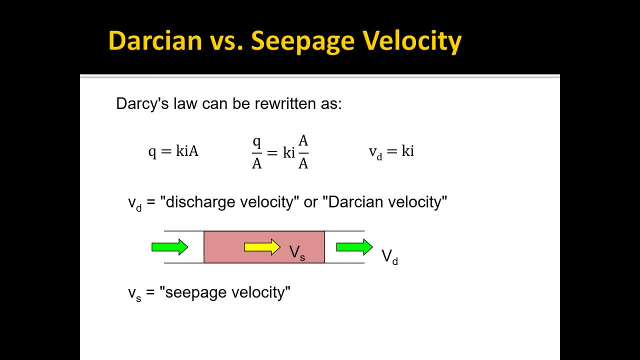 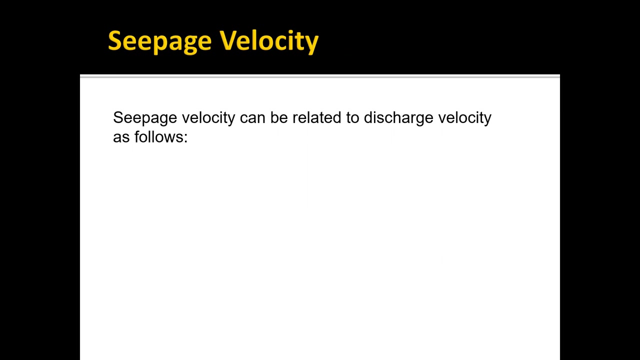 So if you take that same volumetric flow rate and you push it through that much smaller cross-sectional area, you're going to get the seepage velocity should be greater than the Darcy velocity. Okay, and now let's drill down into this a little more closely. So how do we determine the difference between the seepage velocity and the Darcy velocity? 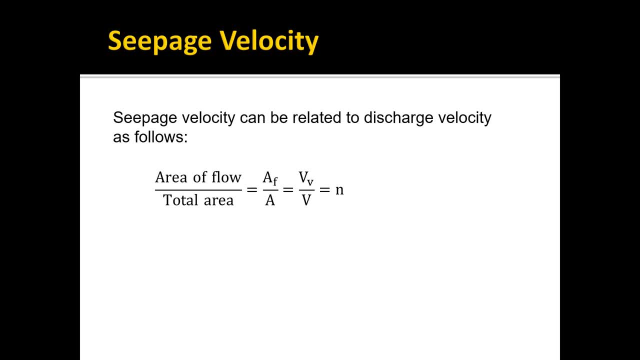 So if you look at the ratio between the area that the flow occurs, the area of the pore space in the soil cross-section, and divide that by the total area, that should be equal to the volume of the voids in the soil divided by the total volume. 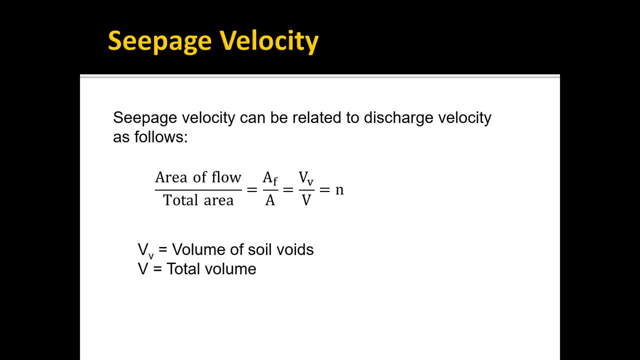 And that. so the V sub 2 is equal to the volume of the voids in the soil divided by the total volume. So V is the volume of voids, V is the total volume, and this term, volume of voids divided by total volume, is what we call porosity. 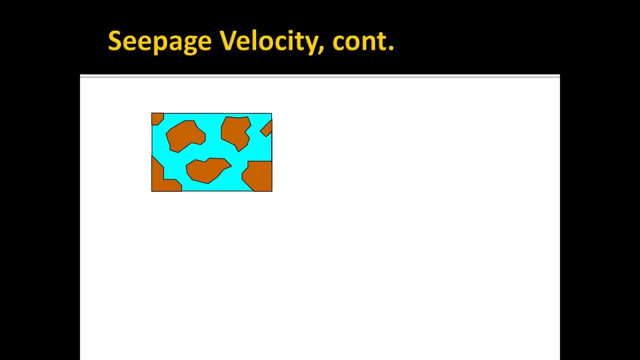 And based on that, if we take a look. so let's say this is our cross-section of the soil. The blue represents the pore space filled with water and the brown represents the, The rock or the soil. So the porosity N is equal to the blue area divided by the total area. 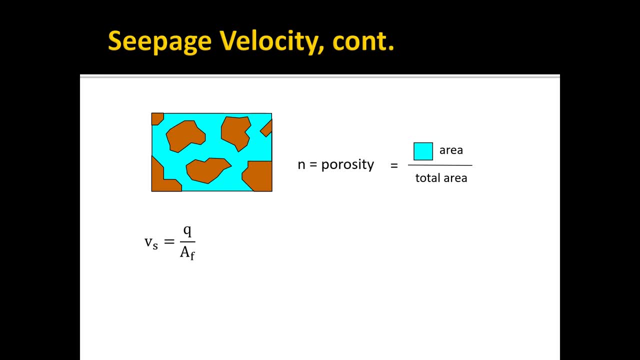 Therefore, if we say the seepage velocity should be equal to the total flow rate, Q divided by just the area of flow, the blue area, And if we take this equation and we We multiply the top and the bottom by the total cross-sectional area A, the Q over A term represents the Darcy velocity. 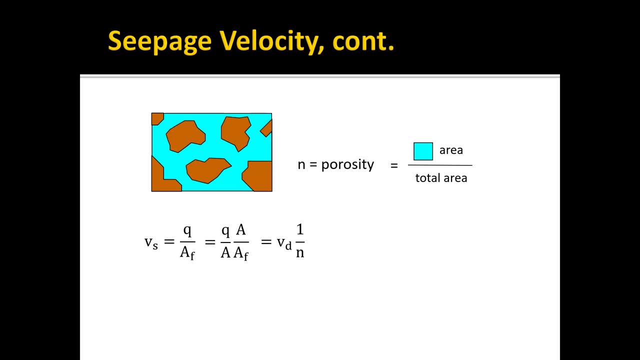 So the flow rate divided by the total area and then the area, the total area divided by the area of flow, is like the inverse of porosity. If you take the air, the blue area divided by the total area, you'd have porosity. 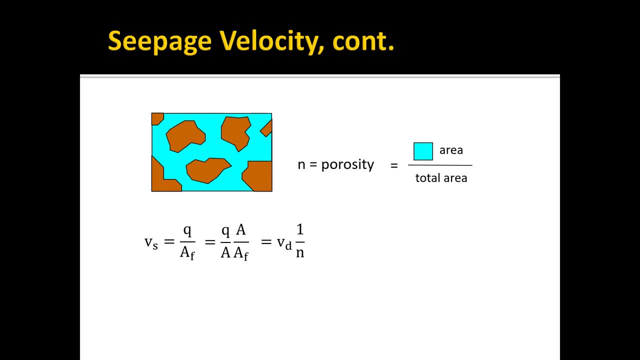 So if you flip that upside down, you get One over the porosity. Therefore, there's a very simple relationship between seepage velocity and Darcy velocity. To get the seepage velocity, you simply divide the Darcy velocity by the porosity of the soil. 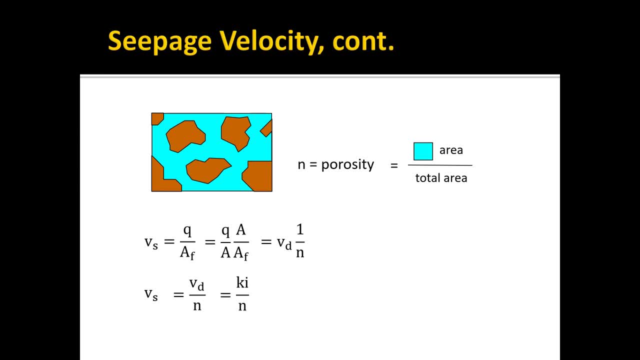 And so another way to write Darcy's law: VD equals KI, but VS equals KI. So we've got this expression here and we're going to estimate the seepage velocity. So we're going to do this with KI divided by porosity. 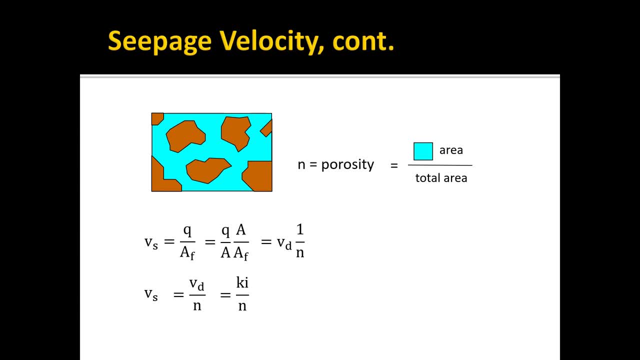 So we now have a way to get an estimate of what the seepage velocity should be. So this is really important. When we apply Darcy's law, we've got to remember to divide by porosity to get. If we're back calculating the velocity, it's important to divide by the porosity so that we're getting the actual seepage velocity and not the Darcy. 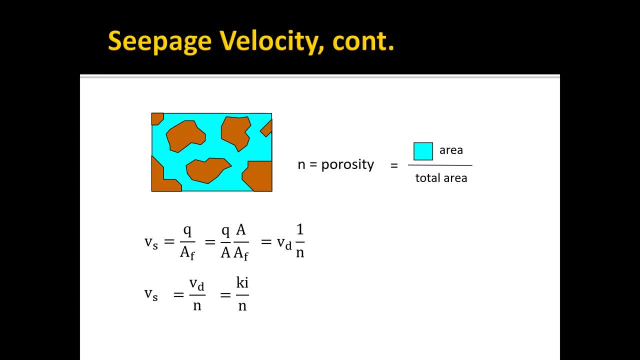 The Darcy velocity by itself doesn't necessarily have a useful physical meaning in flow through porous media, but the seepage velocity certainly does. Now let's look at some of these ratios. here In this table I've listed some porosities. 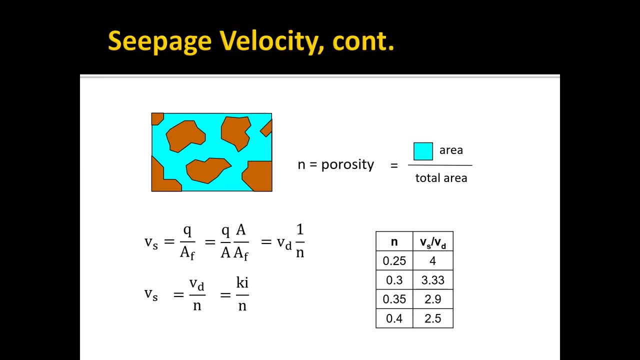 I probably should have started this at a lower number. In fractured rock you can have porosities down on the order of, you know, 0.01, 0.02, 0.05, something like that. Actually, 0.25, 0.3 would be relatively typical porosities for sand or gravel. 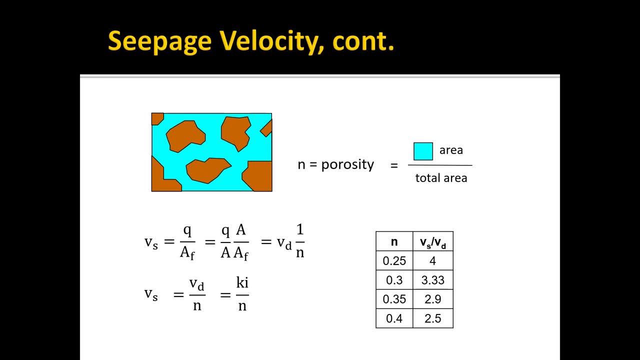 0.4 would be very high, And you can look at the ratio For those particular porosities. if you look at the ratio of seepage to discharge velocity, we're talking, you know, a pretty significant difference, And so that's why this becomes important. 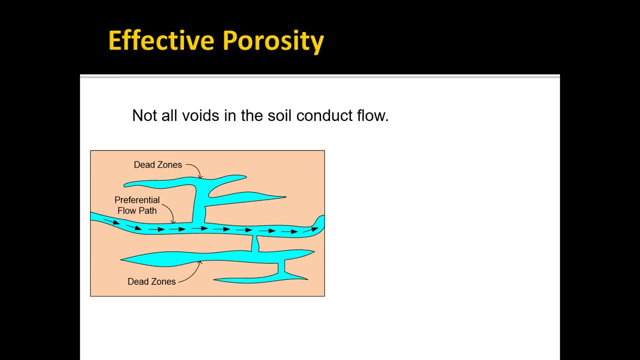 Now this gets a little more interesting. It turns out that we need to modify this one more step because not all of the voids in the soil necessarily conduct, So we were talking about the area of flow as part of that gross cross-sectional area. 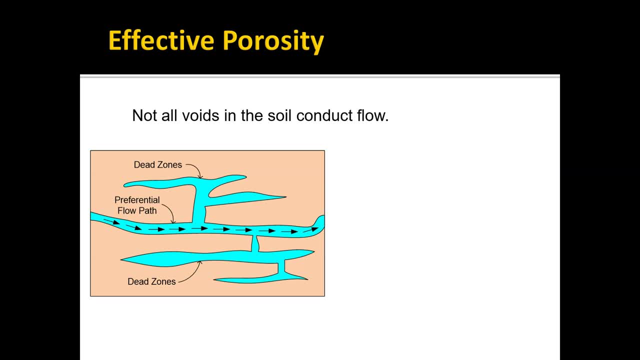 Well, let's suppose you have fractured rock And I've got some really big fractures here that aren't very realistic, But just to illustrate the point. But theoretically you could have some preferential flow paths and then some kind of dead zones where it's filled with water. 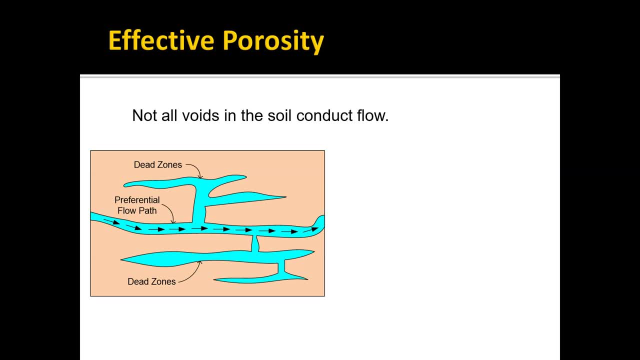 but not much flow, And that's what we're talking about here. So if you take the entire porosity and calculate the seepage velocity using the entire porosity, you would end up with a seepage velocity that's too slow. 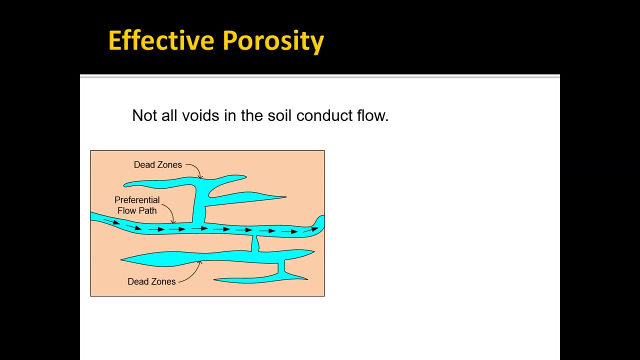 If the actual area of flow is smaller, you're going to have a much higher velocity or a bigger differential. So there's a new term we call, we use, which is called effective porosity or n sub e, And that's equal to a f over a, where a f is the actual area of flow. 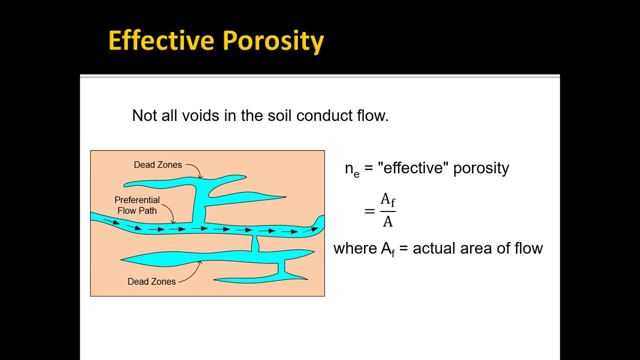 It could be some fracture of the void space. The poor, the saturated water area of your cross section is just what fraction of that actually conducts flow And therefore the the most appropriate way to represent seepage velocity is K? I over n sub e, where n sub e is the effective porosity. 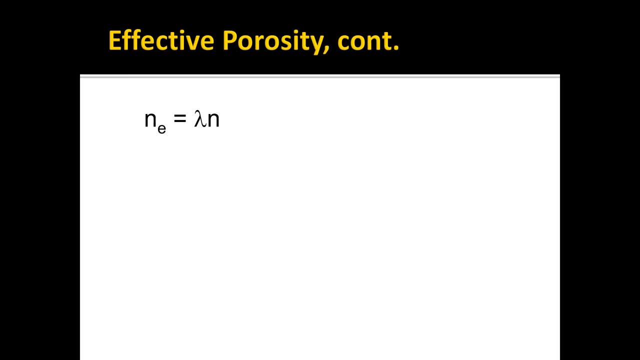 So, if you think about it, effective porosity is going to be equal to some fraction of the total porosity. Um, you can. sometimes it's written like this, with a lambda, where lambda is the effective porosity factor, We determine it's. 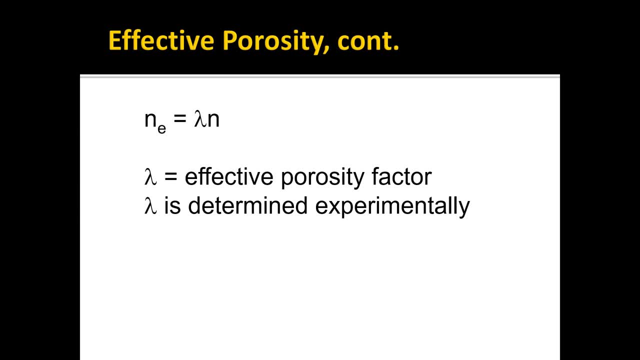 experimentally, and it varies between zero and one. if you have relatively clean sands and gravels, the effective porosity will be uh, it'll be approximately one, meaning all of the voids in the soil are active in conducting flow. However, 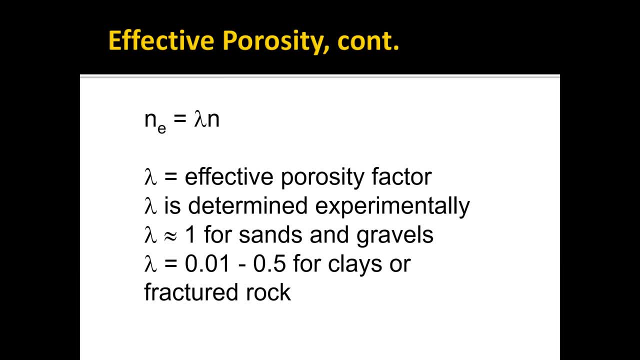 it can be quite small. I mentioned fractured rock earlier. Uh, the effective porosity factor could be as low as one percent. Um, that is a typo. Well, no, that's that's. that's, that's okay. 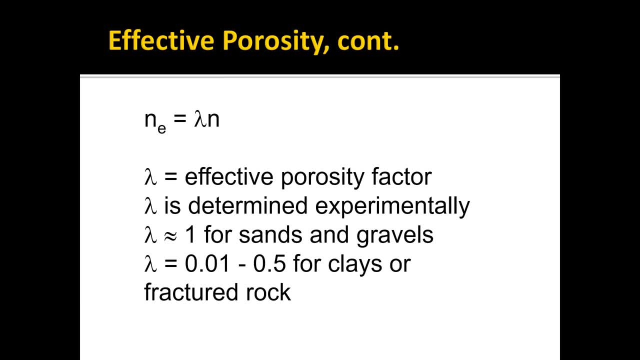 Uh, point, oh one, maybe up to point five for clays or fractured rock, but it can be quite small. So there are going to be a number of times in our exercises and our homework We're going to be calculating. We're going to be calculating the seepage velocity from Darcy's law. 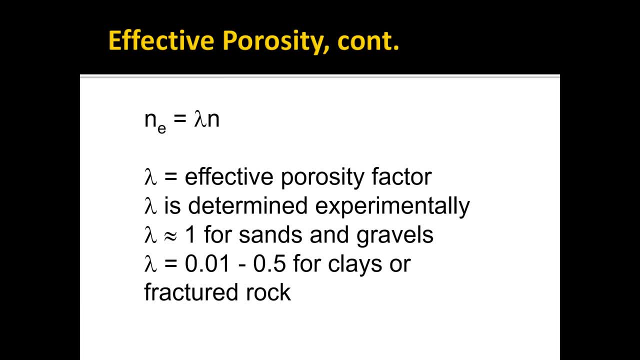 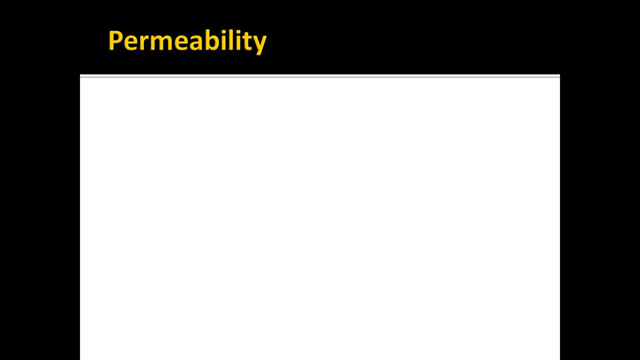 And when we do so, we're going to, uh, use effective porosity, which is something that I'll be providing to you when you need it. Okay, Finally, um, a couple more things to look at and understand, Um. 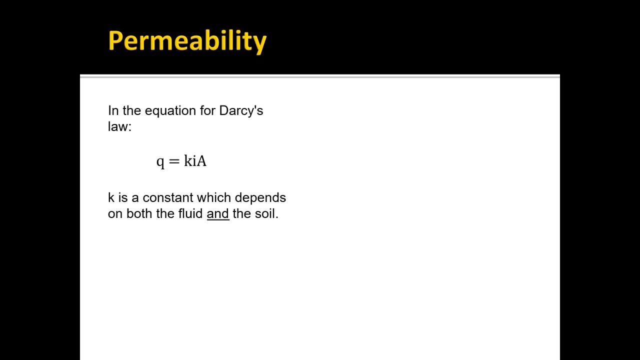 we've been using the term hydraulic conductivity, uh. in the equation for Darcy's law, Q is equal to KIA. The term K is a constant in which we determine experimentally or estimate it, And it actually depends on both the fluid and the soil. 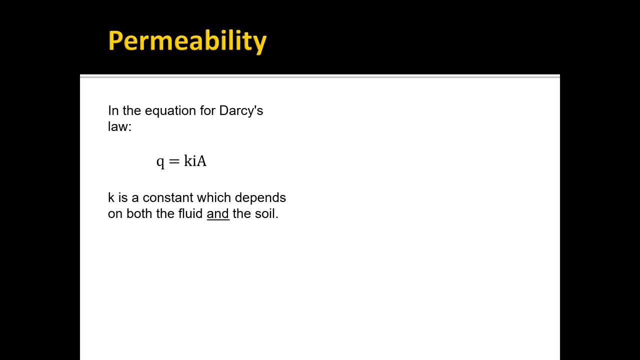 That is why we often call it hydraulic conductivity. Hydraulic implies water. However, you can rewrite Darcy's law in this form: Q is equal to minus capital K, gamma, F over mu, times DHDX, times uh times a minus the minus DHDX. 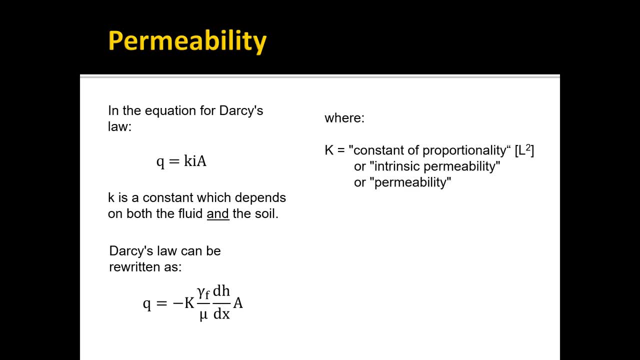 Again we're back to the derivative form. A is the cross-sectional area, But in this case we've got a different K instead of hydraulic conductivity, with units of uh length per time. This is the QF constant of proportionality in. 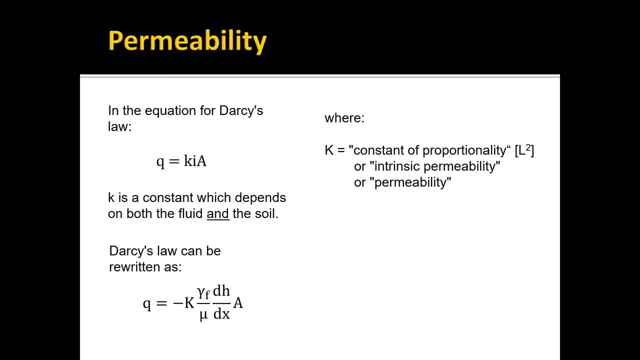 or often called the intrinsic permeability or the permeability, And it has units of length squared And it is based on the soil properties only. So where does the, where did the fluid properties come in? Uh, that comes in in the gamma F. 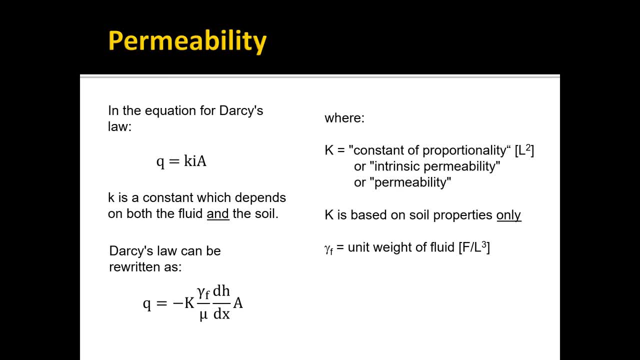 which is the unit weight of the fluid, which is uh. force per length cubed, And um mu is the viscosity of the fluid. mass times, length over time. Uh, so if you look at this equation in the lower left corner of the slide and compare it to: 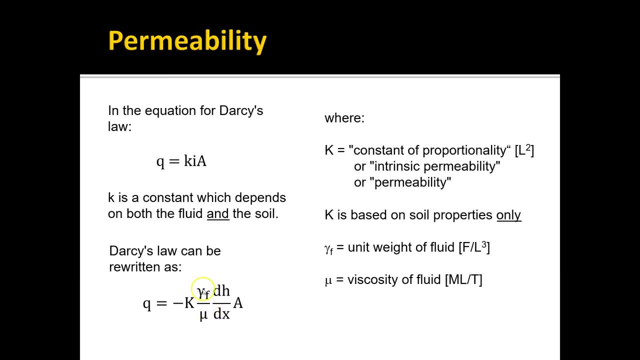 the equation we saw earlier. what's happened is we've inserted, instead of a single lowercase, K, uh, we now have K times gamma over mu And therefore um, as long as you use the proper unit, weight of the fluid and viscosity. 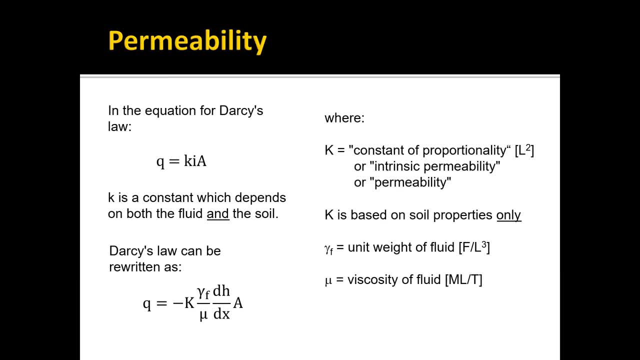 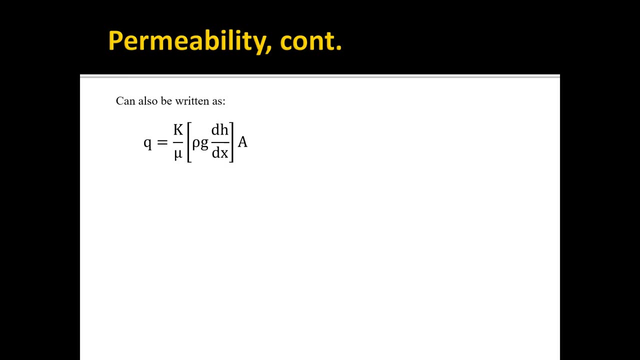 uh, you could, uh, uh, you could derive uh. or you could switch back and forth between hydraulic conductivity and um and the intrinsic permeability form, So um. this can also be written in this form instead of unit weight. 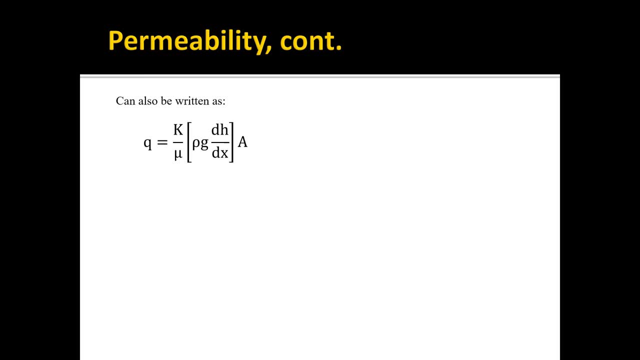 we have density and gravity. Um, I think I'm missing a minus sign here. This should have a minus sign in it. Um, because we're still using the derivative form, And this form is used, uh, among other places, but primarily in the petroleum industry. 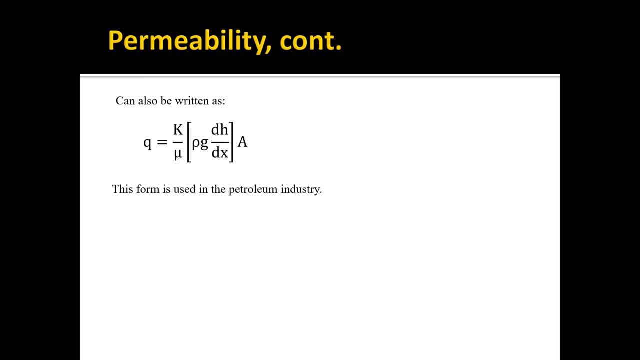 And why do they prefer this form in the petroleum industry? Because they're often. sometimes they're dealing with water, but they could be dealing with natural gas or crude oil, um, or fracking fluid that they put in to um, to. 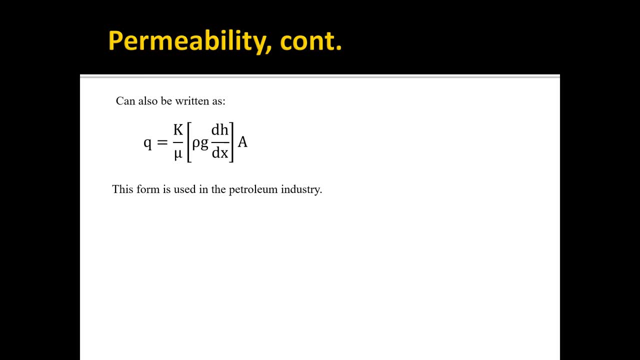 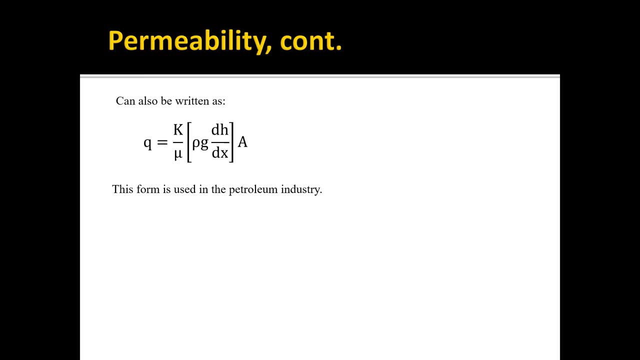 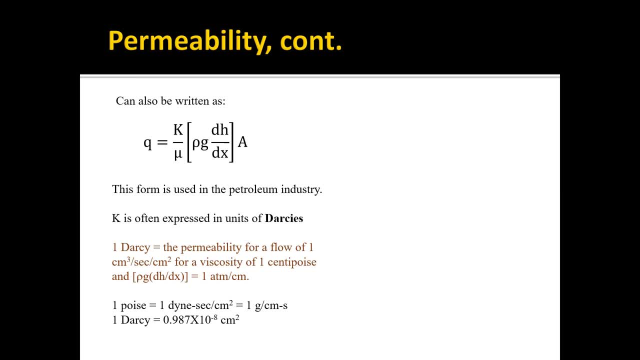 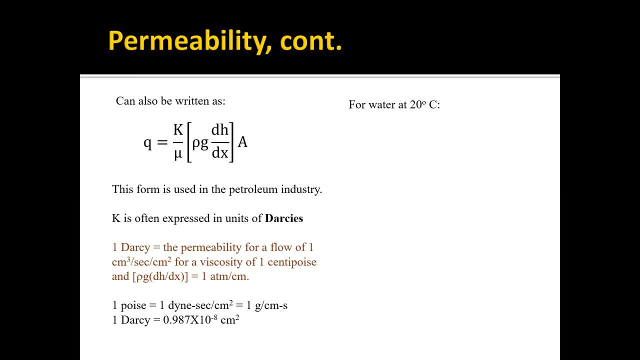 water at 20 degrees centigrade. the temperature of the water controls its viscosity and density. so we could calculate with these given values of viscosity and density and so forth. that's the gravitational coefficient. there we can come up with a, uh for an for a hydraulic conductivity. 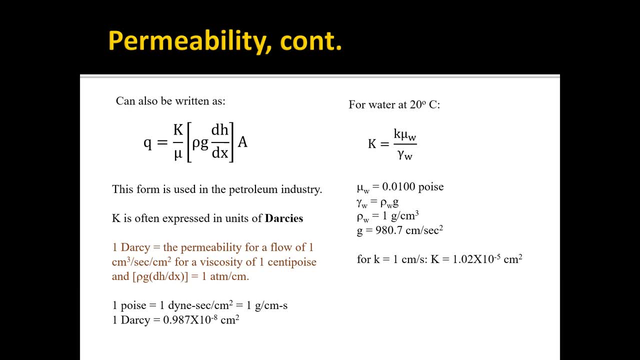 that would be one centimeters per second. you end up with the intrinsic permeability of uh 1.02 times 10 to the 5th, 10 to the minus 5th centimeter squared. so this alternative form of darcy's law that is based on intrinsic permeability and 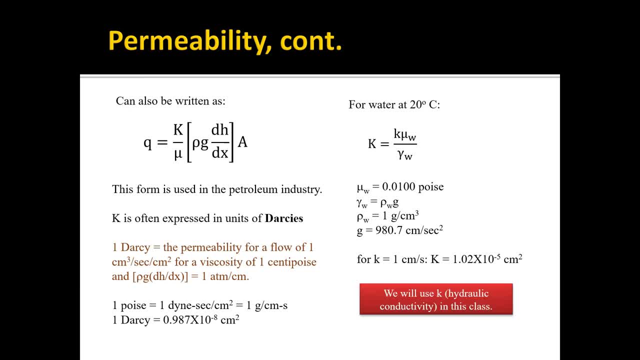 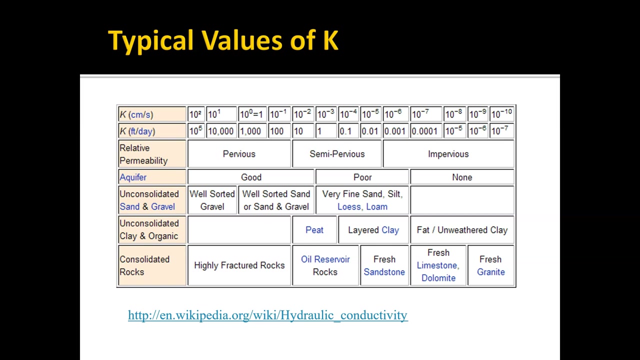 including the fluid properties is just for your information. in this class we're dealing with groundwater. therefore, we will use hydraulic conductivity. this was presented as background in case you see this other formation of darcy's law. finally, um years ago i taught this course and- and in the student comments, somebody 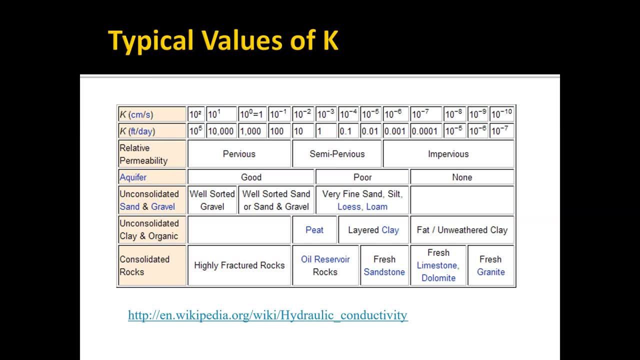 said, i took the whole course and i still don't know how to estimate hydraulic conductivity. so i'm trying to be a little more proactive and try to give you a sense of what a reasonable range of hydraulic conductivities are for different types of soil. this is a fairly standard representation. 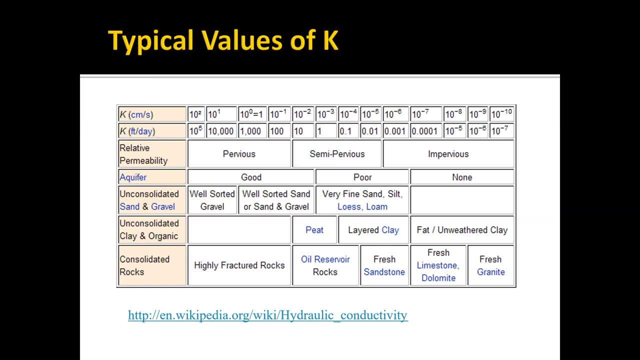 of how hydraulic conductivity varies, and so the two most common units we use for hydraulic conductivity and metric units. we often use centimeters per second and in english units we often use feet per day. why? why seconds for one and days for the other? i'm not sure, but this 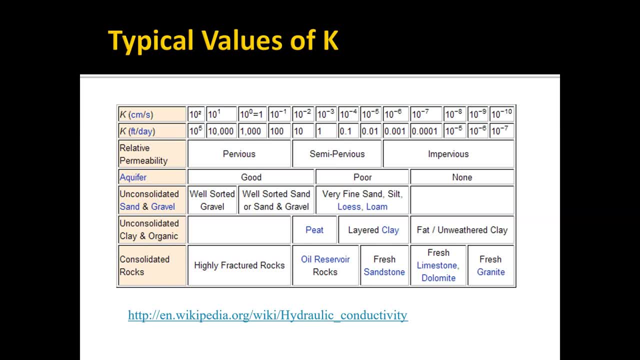 these are the two most common uh ways we represent hydraulic conductivity in each of those, and they differ from one another by a factor of about three orders of magnitude roughly, and so you know, looking at feet per day, what we're talking about with this say generally. let's look at this term, it says good, aquifer. so 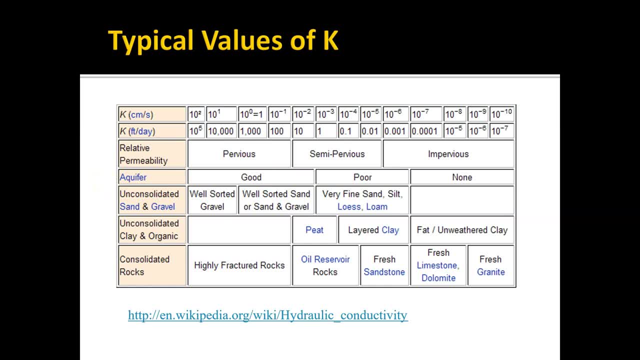 a good aquifer is something where- uh it's gonna, the water will flow through it quite easily and we can pump water out using wells without expending too much energy and we can get a good draw. so you, you need to have a hydraulic connectivity of about one or greater. 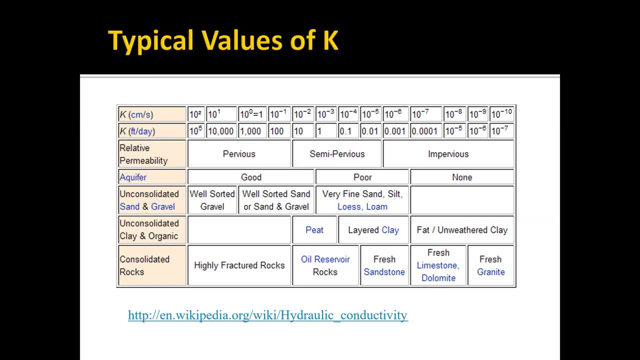 common to have hydraulic conductivities- 10,, 20,, 50,, 100, 200 for an aquifer, And then, likewise, you know we're talking about 0.01 centimeters per second or greater, all the way up to you know, maybe one centimeter per second being a more typical range, I did. 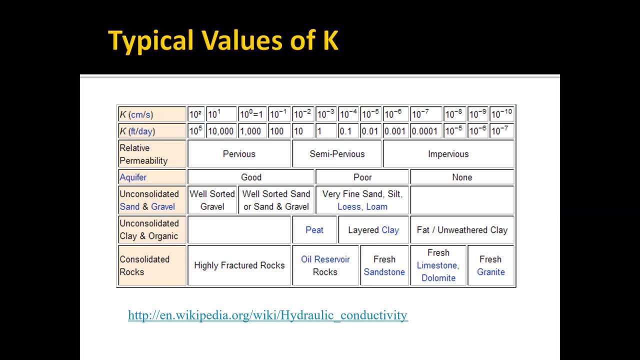 encounter an aquifer in Hawaii once that had hydraulic conductivity of 10,000 feet per day, which is kind of what it was really: porous, igneous rock lava, basically near Pearl Harbor in Hawaii. So sometimes you'll see super high hydraulic conductivities And 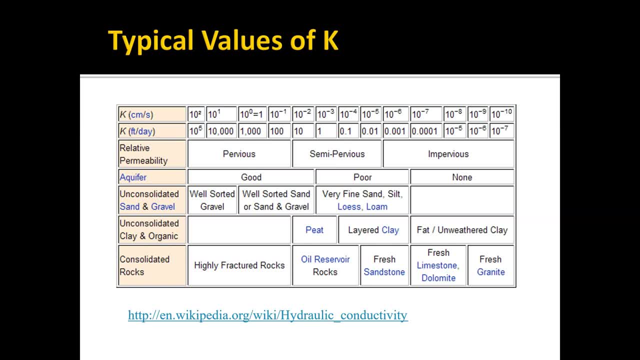 then another benchmark for me, if you look down the scale here, if you're ever designing a landfill or a liner for a water containment facility generally, we like to see a compacted clay liner be on the order of 10 to the minus 7, 10 to the minus 8. 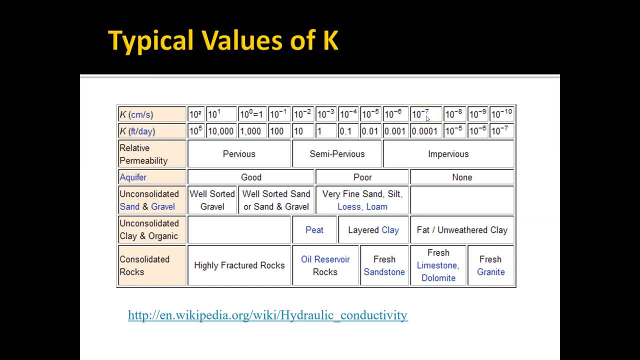 centimeters per second And if you have a foot of standing or about a, you know, a third of a meter or a foot of water standing on top of a clay liner, it would take about 30 years for it to get to travel through the liner.